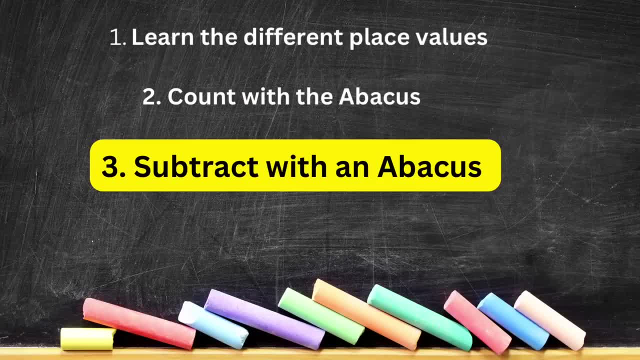 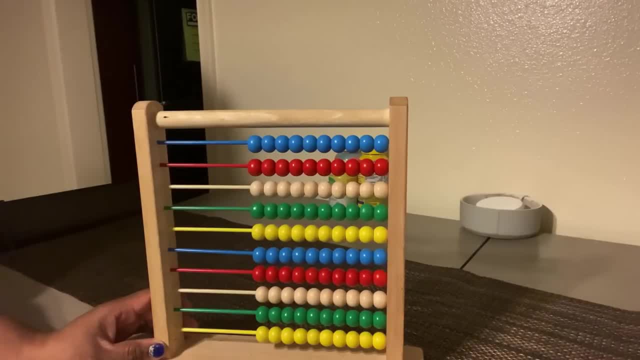 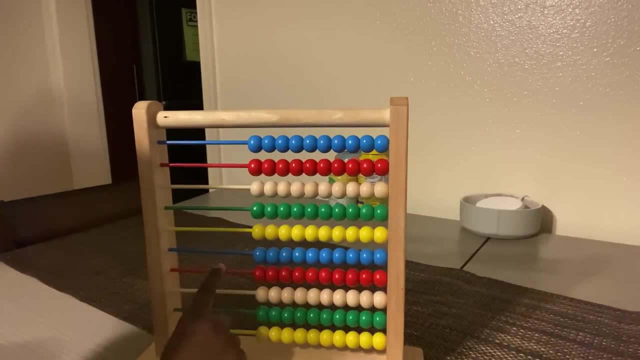 Hi everyone, we're loading Subtraction with the Advocates and, just in case, if you do watch our edition one, this is the ones place. this is the tens place. this is the hundreds place. this is the thousands place. this is tens place. this is the ten thousands place. 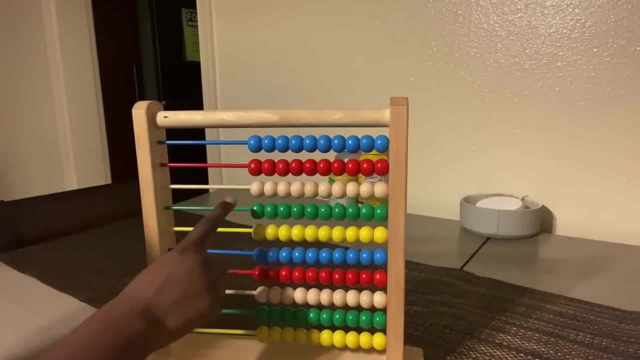 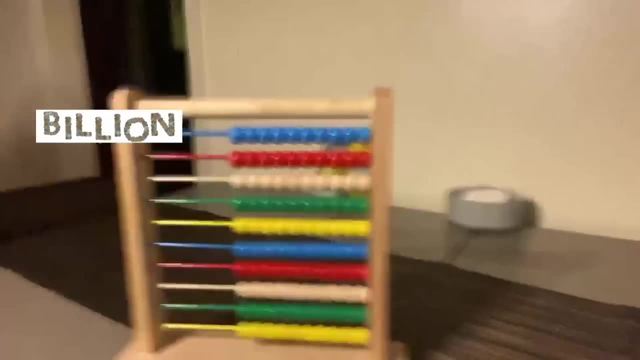 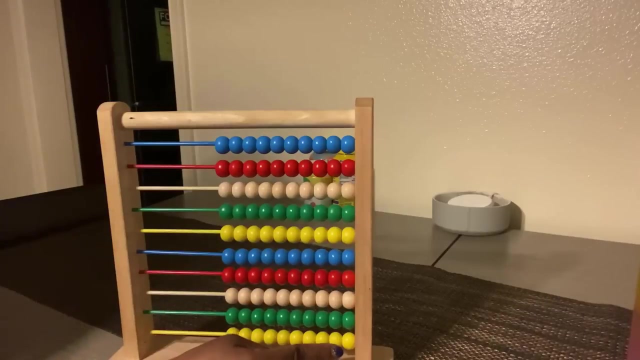 this is the hundreds thousands place. this is the one millions place. this is the tens millions place. this is the 100 millions place. right in the next section. we'll count using the abacus. what is this row? those are the ones place. so how many is here ten? how many is here those? 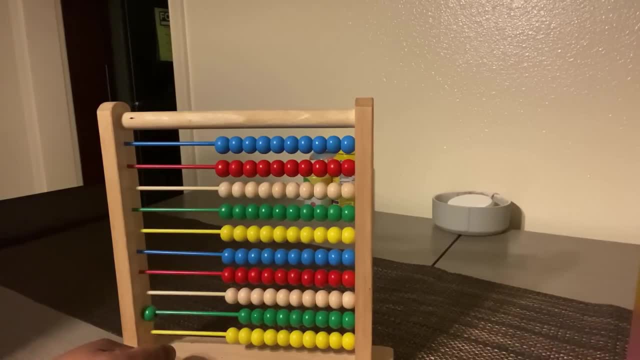 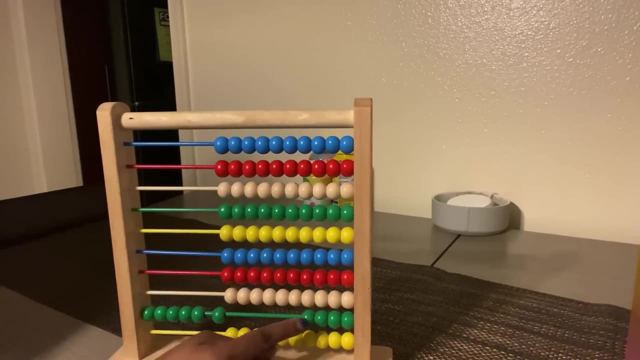 are the 10th place. so what is this? um 10, 20, 30, 40, 50, 60, 70, 80, 90, 100, right? so let's go back to this one. so what is this? one, two, three, four, five, six, seven, eight, nine, ten. 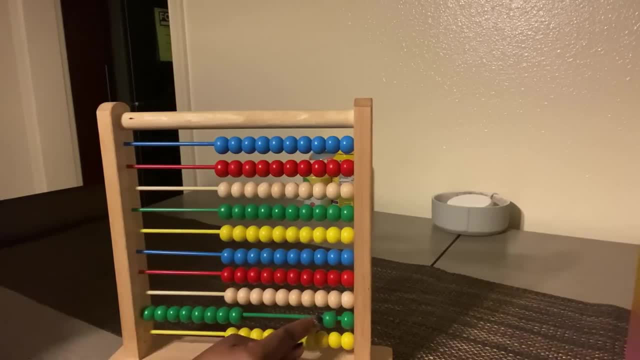 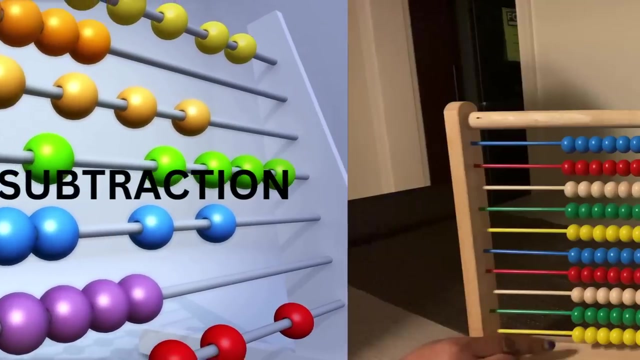 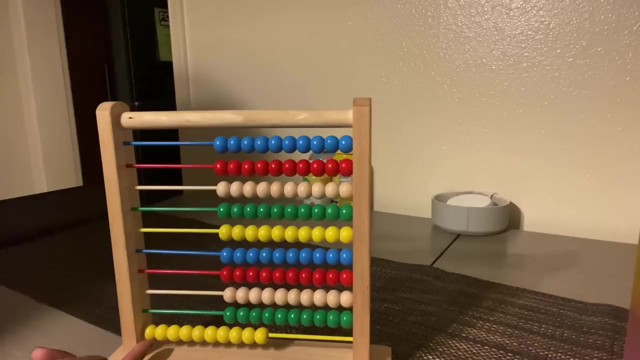 10 right: 10, 20, 20, 30, 40, 50, 60, 70, 80, 90, 100. now it's time to subtract. so simple subtraction. let's say we have how many is here? 10, 10 minus 1 equals. 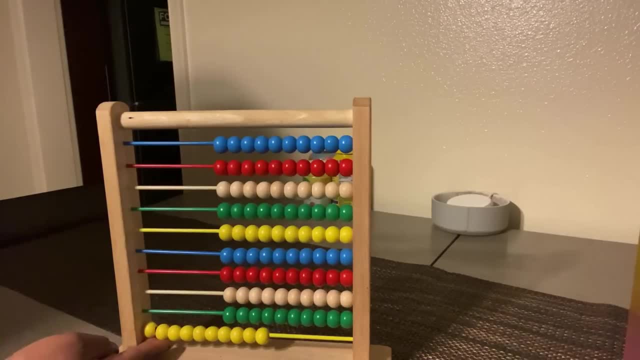 10. so now i have again: 10 minus 2 equals 10. minus 2 equals 8. okay, now we have 10 minus 3 equals. so count one, two, three, four, five, six, seven. okay, so we have 10 minus 10 percent. minus four: equals that equals six. count one, two, three, four, five, six. great, now we have again ten minus five minus five.